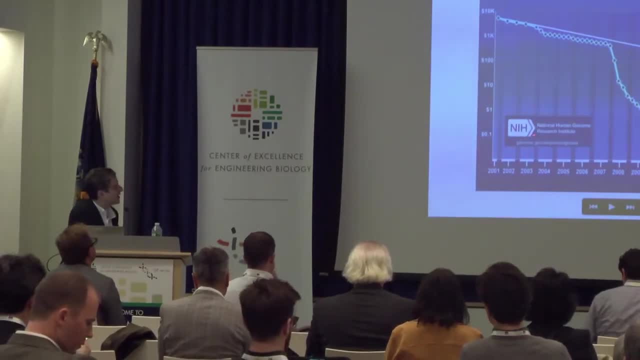 This is a curve I'm sure you've all seen. It's from the NET and the GRI website And it shows the scaling in sequencing data generation which, as you all know, has been amazing, And that's one of the things about DNA sequencing scaling. So until about 2007 or 2008,. this 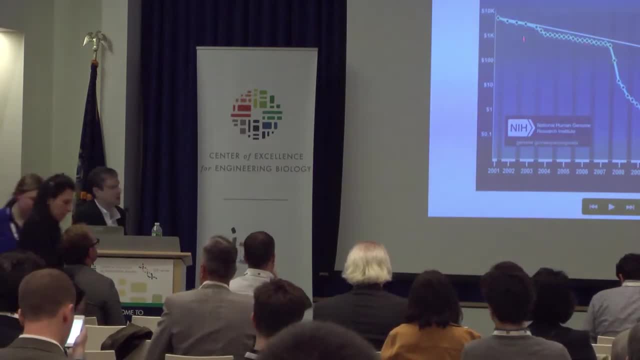 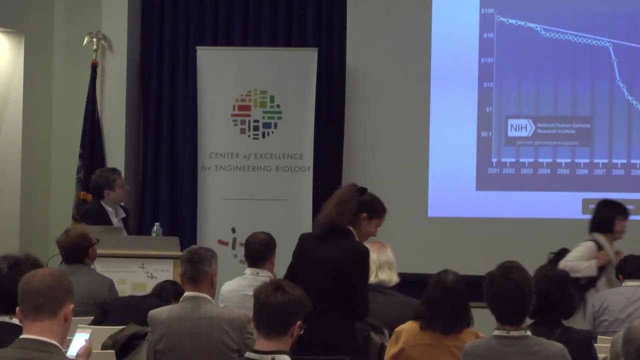 was, of course, scaling exponentially. This is a straight line on a log which shows you the exponential scaling, And it's following the exponential scaling that we've traditionally seen in the computer industry And around 2007,- 2008,, we first had this amazing advent. 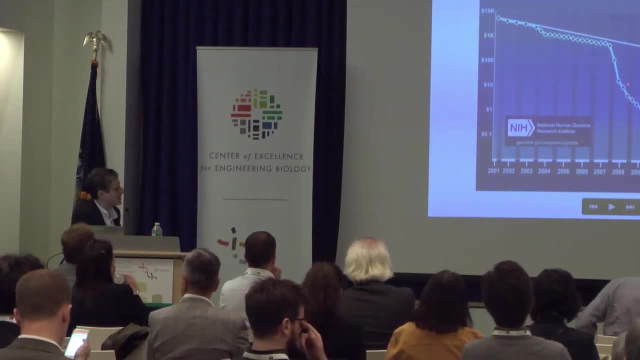 of next-gen sequencing, where we got this exponential scaling, Sequencing became much cheaper and cheaper. And then notice, though, that subsequently we look like we kind of resumed to some degree, paralleling that on Earth or online And for people who have spent. 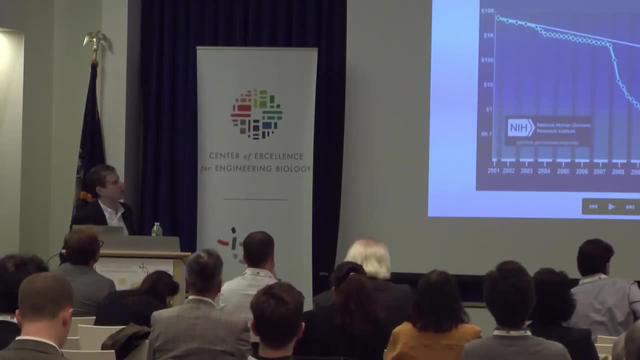 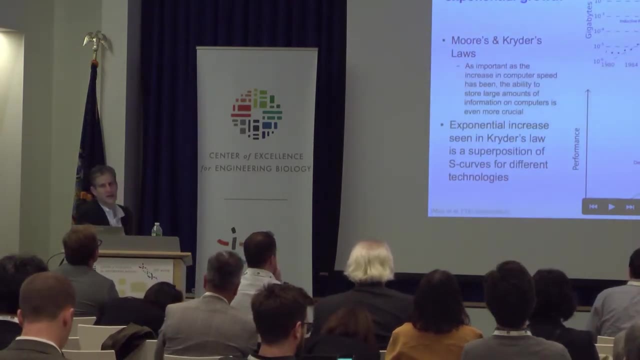 a lot of time talking about. you know, is it scaling? Well, it's not scaling. It's exponential or it's not. How do we think about scaling in the future? I'd like to posit that scaling in DNA generation actually follows what we've studied. It doesn't follow. 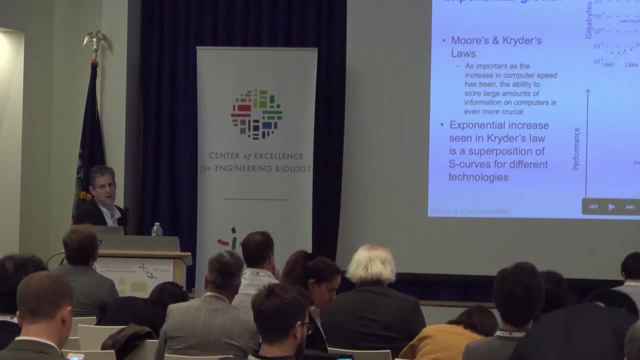 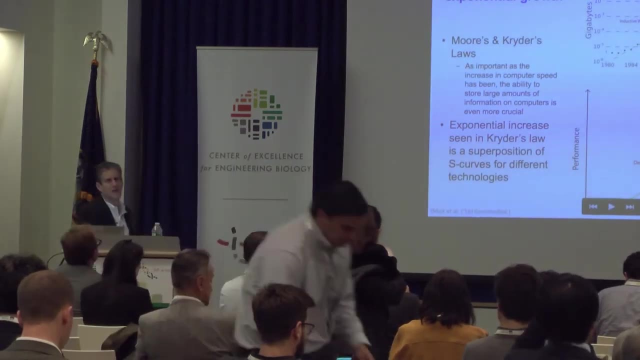 Moore's law. It follows this thing called Prider's law. So what is Prider's law? Well, Prider was the vice president of Seagate And he came up with the scaling law, a very large, permanent type Moore's law, to describe the way fisk tribes get bigger and bigger. 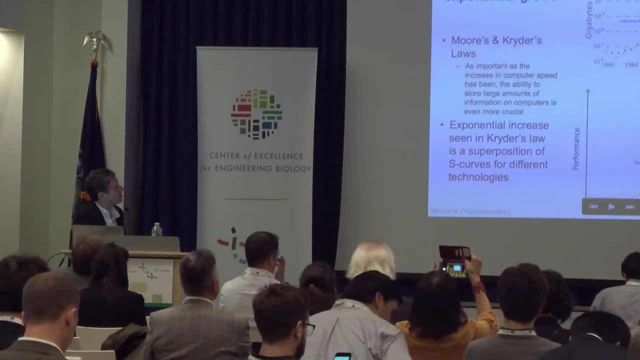 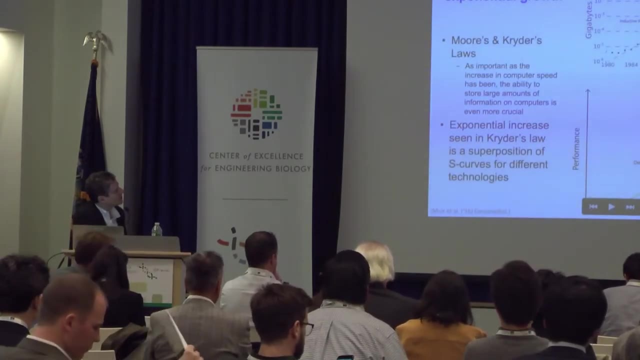 and we can store more corn and produce more corn, And it's an exponential scale, It's like Moore's law. But the key thing that we observed is that this straight line, this exponential curve, is actually made up of a superposition of different S-curves, So each 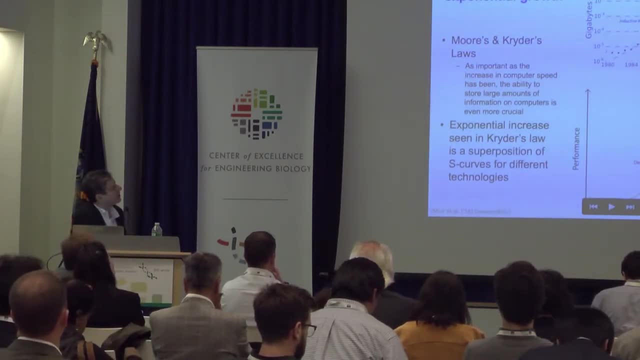 S-curve describes a different technology that's developed, moves forward and then it's phased down, And so, for instance, for this tribe, we have different writing mechanisms that were wheeled in, for instance, during the 1990s, And I would like to posit that that 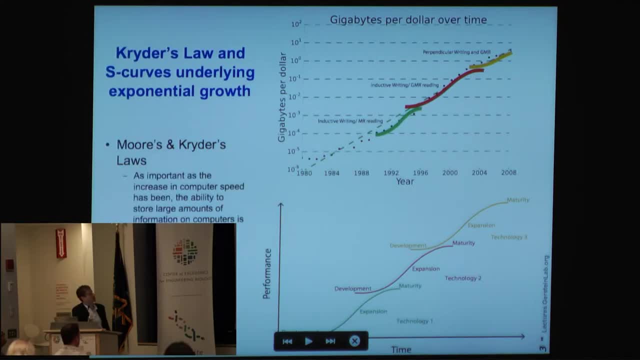 curve that we just saw for sequencing is really important. It's really one of these kind of S-curve-like phenomena And I think that this Prider's law and Moore's law phenomena obviously governs much of what we see in the computer world. 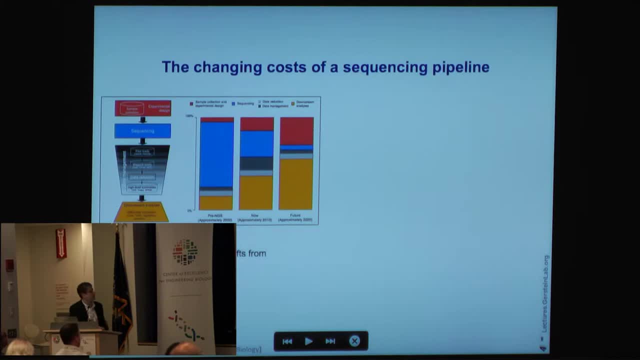 And I believe it also governs what we see to some degree in the sequencing world. So then the question is: how do these two scaling behaviors come together? And this schematic kind of shows kind of how to think about it a little bit. So let's look at the cost in. 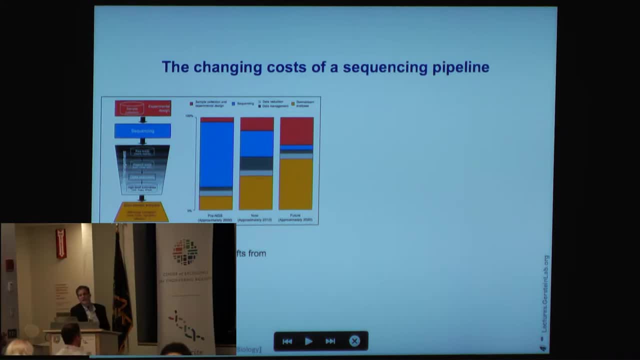 a kind of sequencing experiment, you know around 2000 when the human genome was done. Well, this sort of schematic shows that most of the cost obviously went into the sequencing itself. okay, It's very much like when they first started taking pictures. most of the 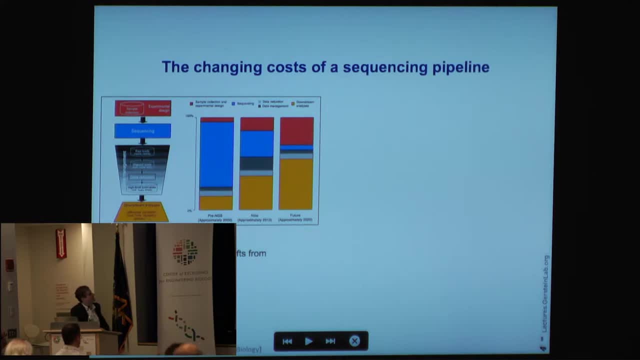 money went into actually the dogger type making the photograph And a little bit went into the sample acquisition and a little bit went into the downstream analysis. Of course, what we've seen with next-gen sequencing is that this blue part has shrunk and of course, 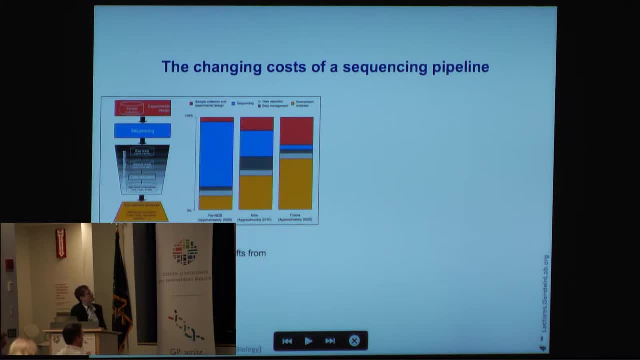 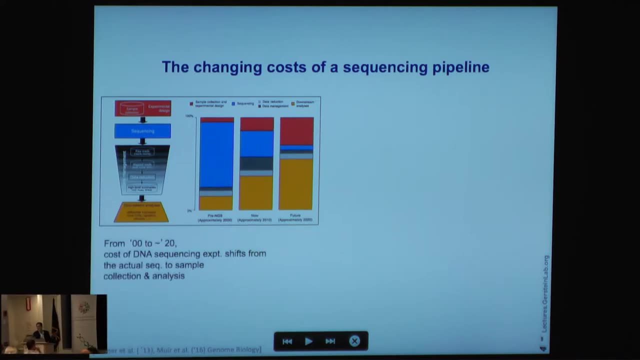 now we have much more of the cost going into the downstream analysis or the sample acquisition, And what we expect to see in the future is, as the exponential scaling of sequencing technology continues, we expect that, essentially, the cost of the sequencing itself to go nearly to zero And when that happens, of course, proportionally most of the cost in one of. 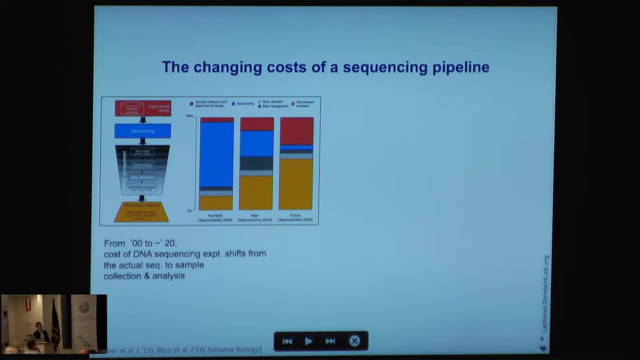 these experiments is going to be taken up by downstream analysis or sample acquisition. It's very much like in photography, where nowadays it costs nothing to take a picture. you can just do that on your iPhone. So what the big thing about photography now is the you know. 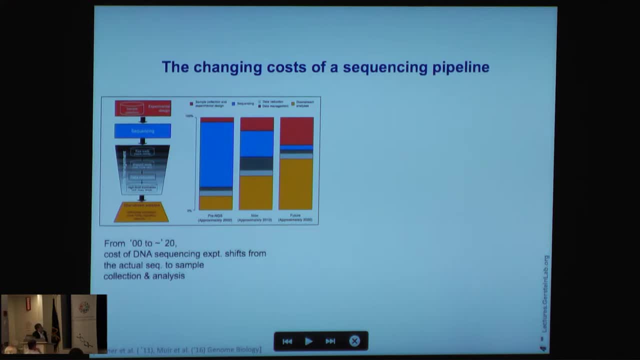 picking the subject, doing interesting things with the photograph. Now I've split up the downstream analysis into what I call pipeline processing, which is storing the data and say, mapping it and doing standard pipeline operations versus kind of more open-ended downstream analysis. And the pipeline analysis actually scales. 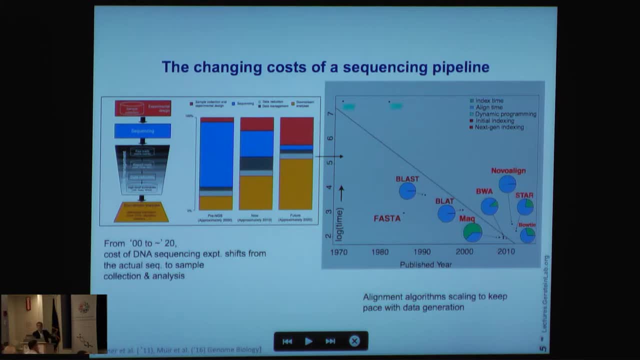 very well with the kind of Moore's Law: increase in disk speeds, processor speeds and so forth. So actually proportionally you don't expect to see it go up that much. And actually one thing that's really neat to see is there's been a kind of parallel Moore's Law. 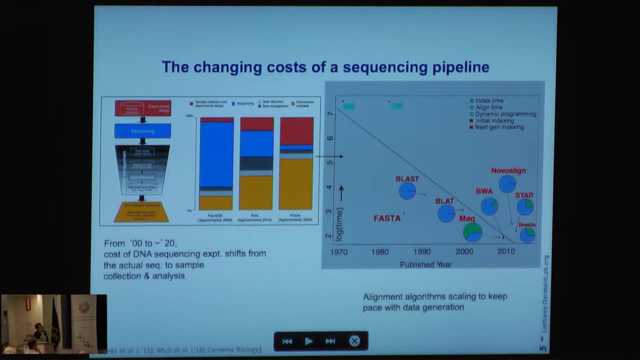 development in the mapping algorithms that people use, for instance in bioinformatics, where, for instance, this picture shows the speed of all these algorithms published on a log graph, And you can see the early algorithms, for instance, that use dynamic programming. 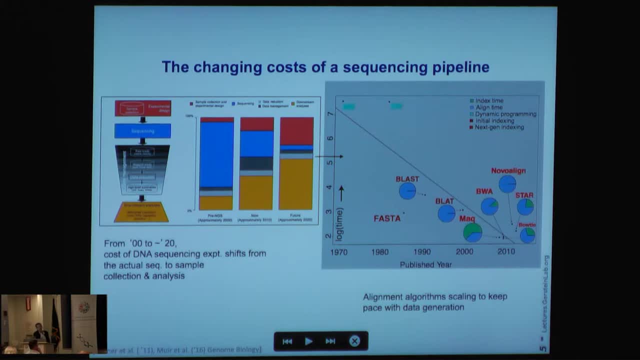 up here the next-gen algorithms such as BLAST that use hashing, and then the modern algorithms such as MAC or BWA that use sophisticated things like the Burroughs-Willow transform, And you can see again a very nice exponential scaling. Of course, the thing that's not 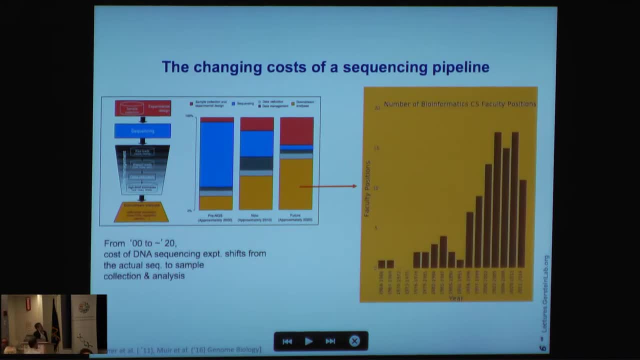 exponentially scaling is this big yellow bubble, which is the downstream analysis, which is completely open-ended, And the reality is it's very important, but we just don't know how to scale it. And because of that, what do we do? Well, we have to hire people and we have to have human brains. 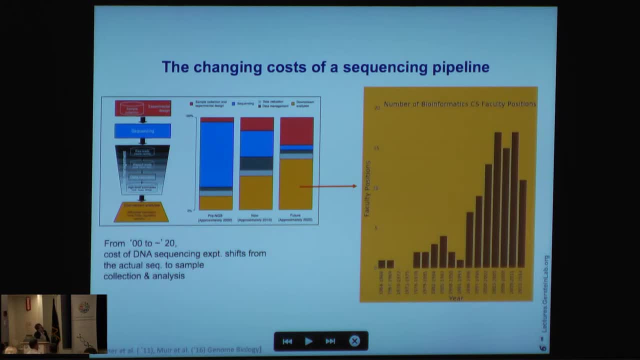 involved and we can't scale that exponentially, And so this, of course, is what that means. This is lots of faculty positions and research positions for people in bioinformatics, which, of course, is very pleasant for me to see many years after living through this world. 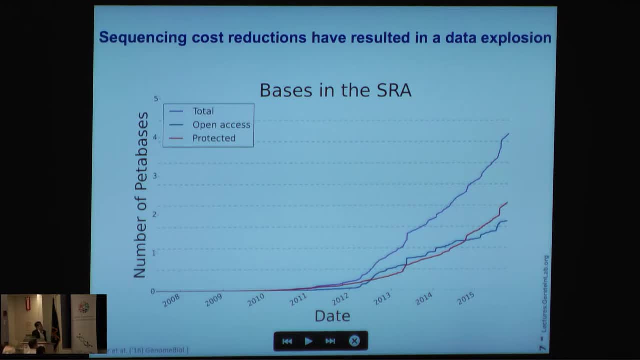 Another thing that the exponential scaling of data generation leads to, of course, is a huge increase in the size of what we're storing in the database. This is a plot you've probably all seen, where we have the number of databases stored in one of the public repositories, the sequence read: repository. 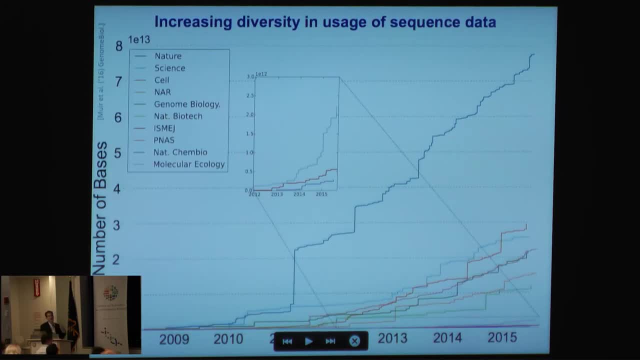 Now, what I'm particularly interested in is we're piling up all these bases, But what's kind of interesting to think about is how the ideas are diffusing through the community, how they're moving through the community, how that's scaling, how our real intellectual output is scaling. 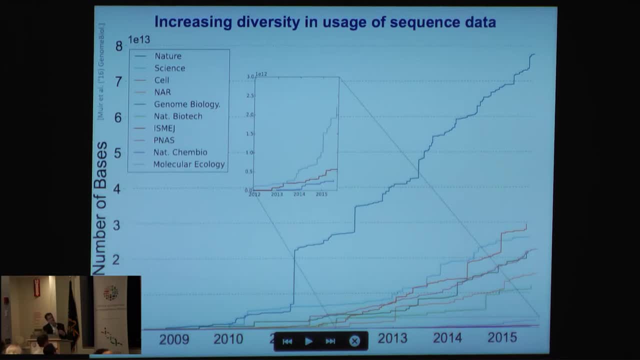 And one way of looking at that is to look at the papers people are publishing in relation to sequencing and look at what subject those papers are in. And so I'll describe a little analysis we do, which is kind of interesting. So this picture shows the number. 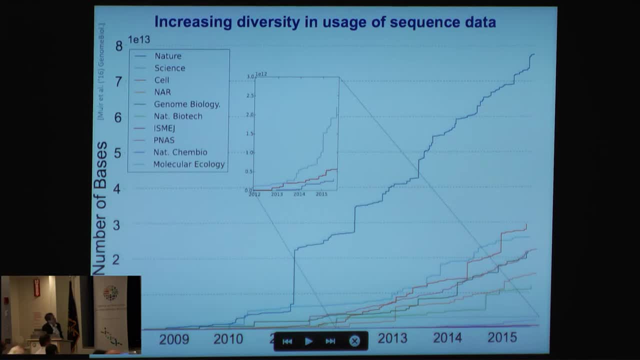 of bases associated with publications in different journals. The different lines are different journals and this line over here this is nature. So this is a huge amount of data that's associated with nature. Nature has traditionally dominated genomics. These lines show, for instance: 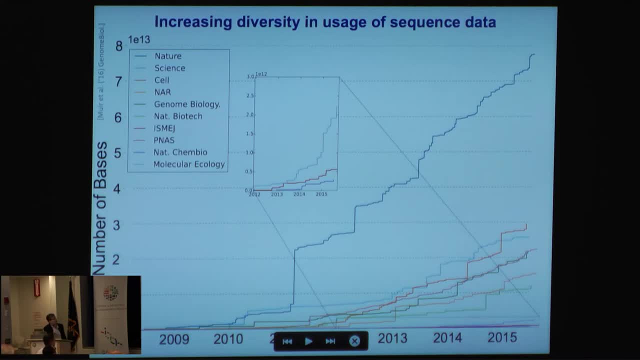 science, cell, other prominent journals, genome biology. But what's really interesting is to look at this down here. These are journals such as nature, chemical biology, molecular ecology. We see sequencing technology and sequencing ideas diffusing into these journals And very quickly I've looked at 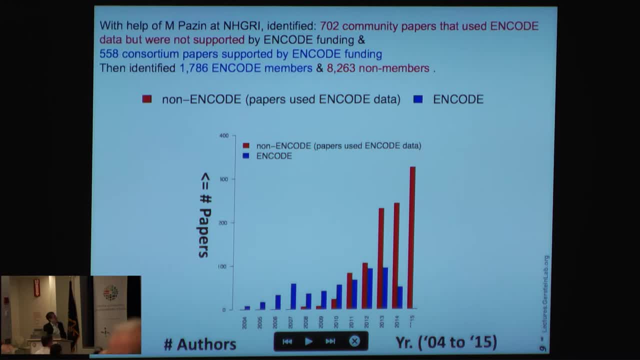 this idea of kind of diffusion of sequencing ideas in a number of contexts. One way of looking at it is looking at what we see happening with various genomics data sets. I've been very involved with this particular data set associated with the ENCODE consortium, where they've diagrammed the 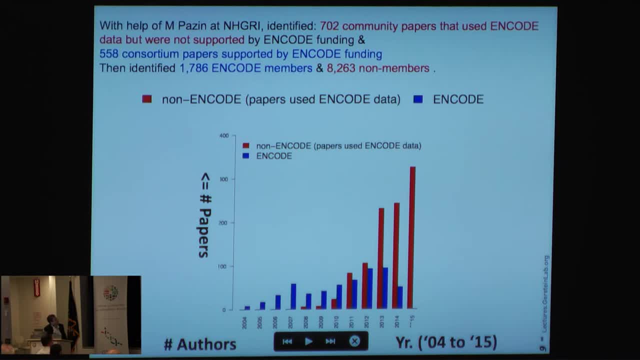 publications in the consortium in blue over time versus those that use the data in red. Obviously, the people using the data rapidly increasing after the data was produced. But what's interesting is because these are publications associated with people, we can actually build the social. 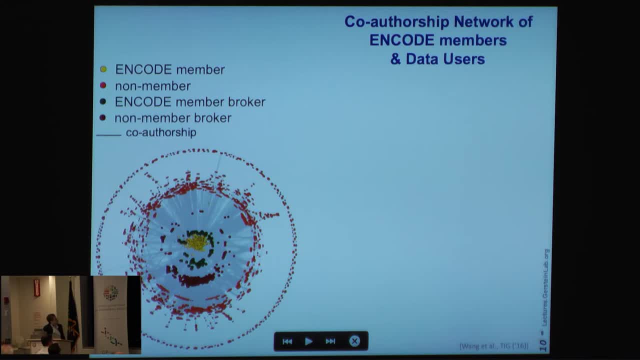 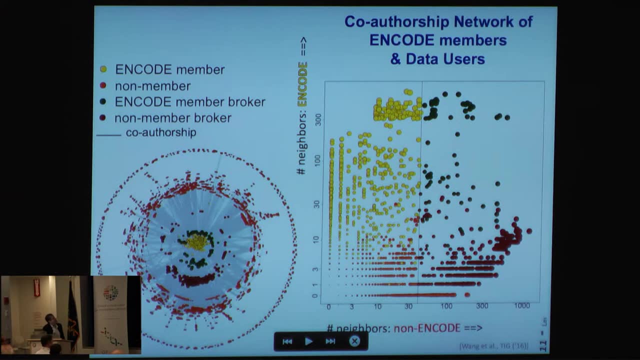 network of how they're used And this shows the social network as of 2014 of people using this data And what you can see. when you look at each person in the network, you can see they break into different groups. There's. 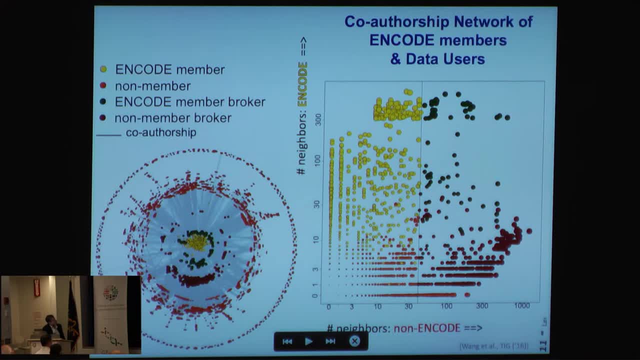 people in the consortium shown in yellow that have high connectivity in the consortium. There's people outside that have high connectivity outside, And then there's a few people that have high connectivity both inside and outside the consortium And we call these brokers. This is this. 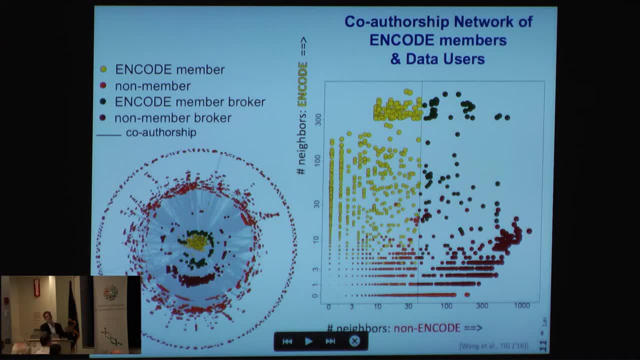 kind of second circle here in this network And these people are really key in terms of the scaling and diffusion of this information outside the little generating group. And what's really neat, of course, is not only can we look at this network, we can actually watch this inner group develop. 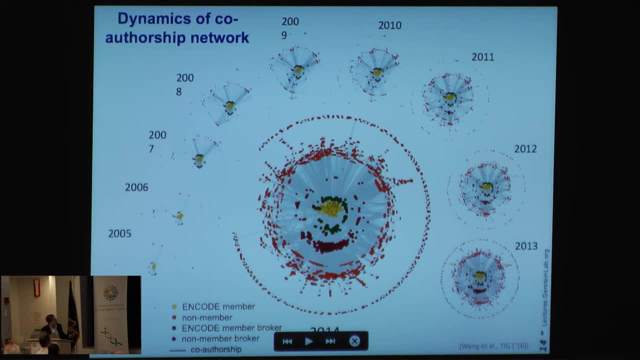 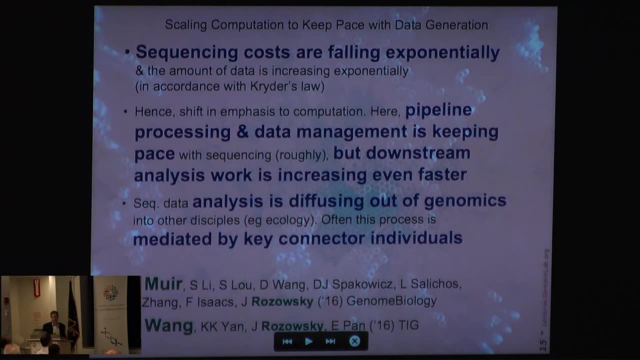 over time from 2004 to 2013.. It's almost like a planetary system you see developing and you can see this diffusion process actually happening. Okay, So I'd like to just conclude. So I've talked to you about essentially two bits of work that have been done in my lab over 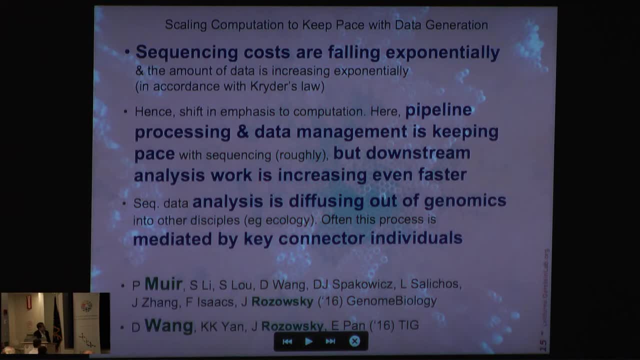 the years. One was this by Paul Muir, who's a graduate student actually with me and Farron, And also Joe Wazowski, an associate research scientist- They worked a lot on the scaling behavior- And Dai-Feng Wang, an associate research scientist. 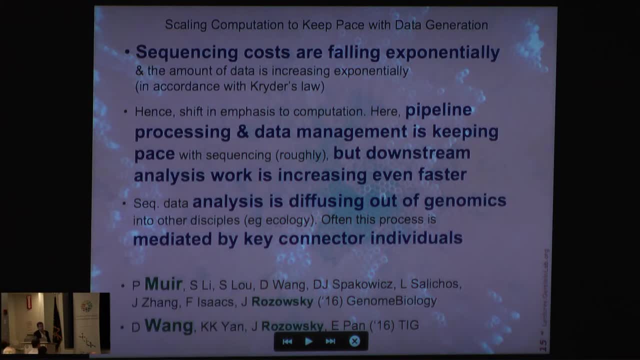 who's moved on to a faculty position, worked on the encode analysis And the quick things I've talked to you about, is the exponential falling of sequence costs. I think the key thing is to keep in mind this Crider's law idea in addition to Moore's. 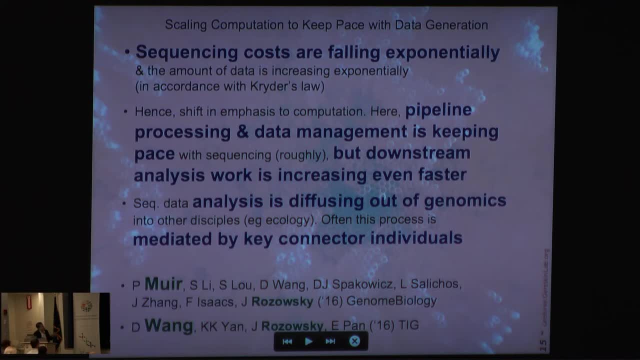 law and how we see, with that, of course, the Moore's law, increase in computing and because of that a fairly constant use of pipeline processing, but this vast expansion of downstream analysis, And then I think a very key thing we also see is this: